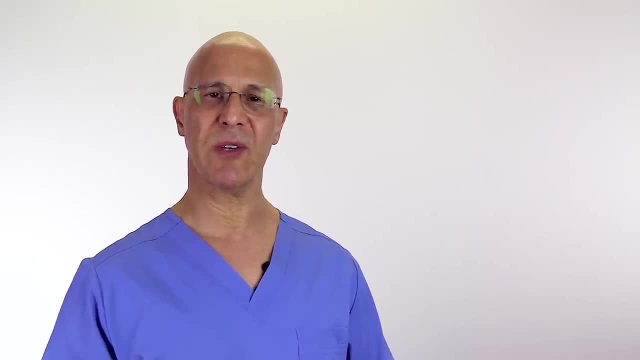 vegetable, the juice comes out. we leave behind the fiber. When we make a smoothie, we put the whole state of the vegetable or fruit in there. we blend it up. The problem, though, with certain smoothies is obviously: what additional things are you putting in? If you're putting in a ton of? 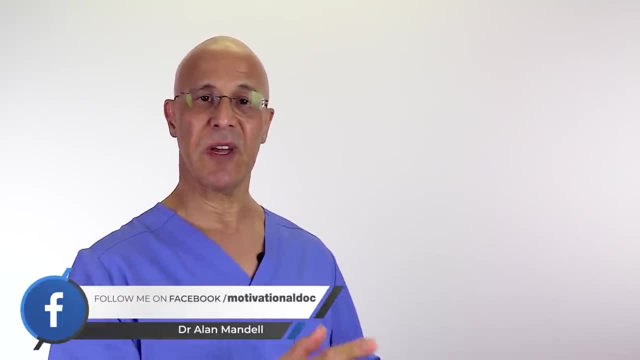 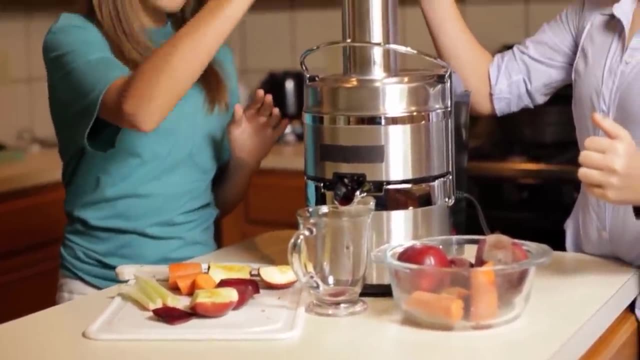 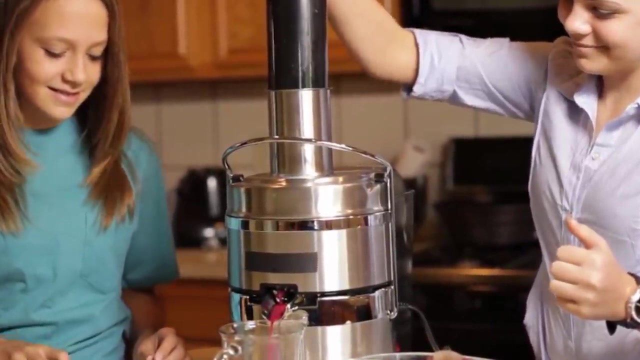 sugar, a ton of honey or other things. that is not good. So when we juice these fruits and vegetables, that pulp, that fiber is all thrown out and that's an extremely important nutrient to us, because very few of us get enough fiber. And, yes, there are plenty of vitamins and phytonutrients in that. 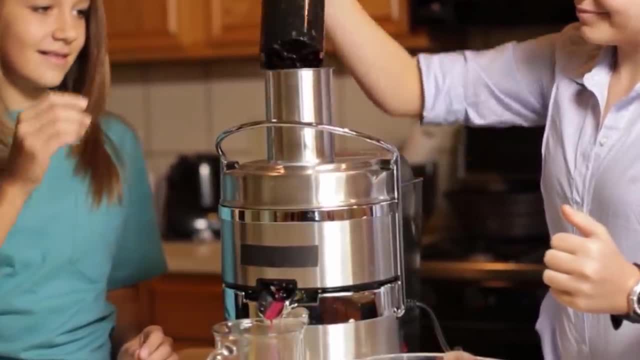 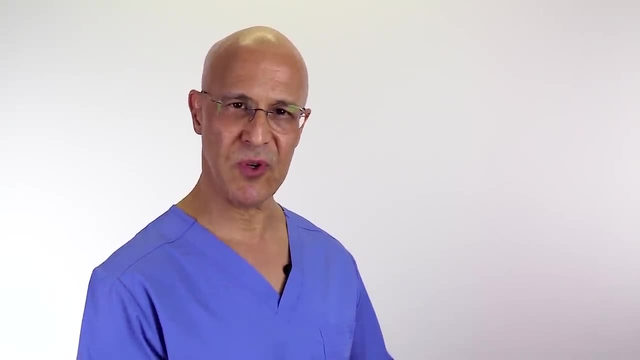 juice, but the fruit or vegetables would also contain those, but maybe not as much. So when you're juicing, it's definitely not good. So when you're juicing, it's definitely not good, But particularly those fruits, which is fructose, that plain fructose that you're drinking, puts a 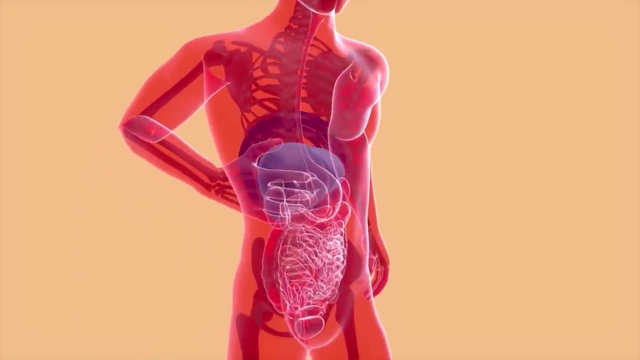 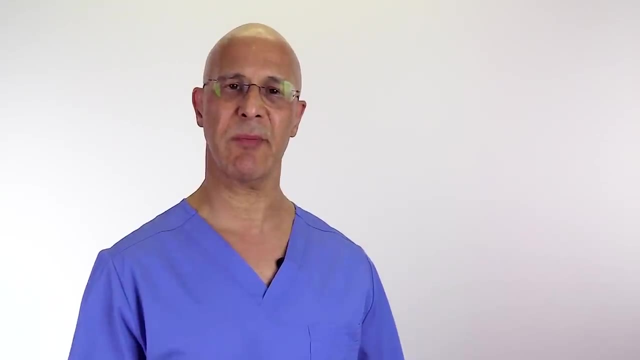 heavy burden on the liver and the liver will get overloaded and it starts turning the fructose into fat. Now here are my defenses. So if we're having more sugar, no fiber, what happens? We spike up glucose, we increase insulin. This abundance of sugar can eventually lead to insulin resistance. 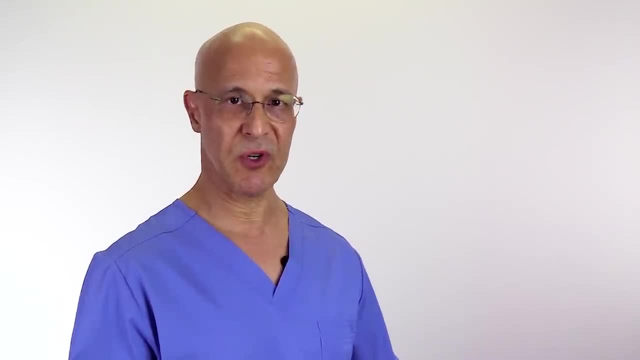 Now the problem here is that the fructose or those sugars are going to be on a higher glycemic scale because there's no fiber. That means that absorption is going to go in really quick and you're going to get that energy and you're going. 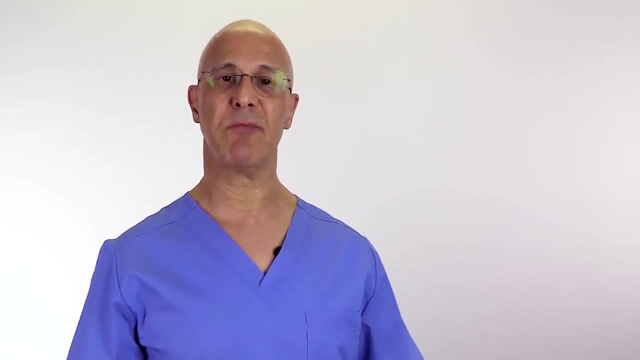 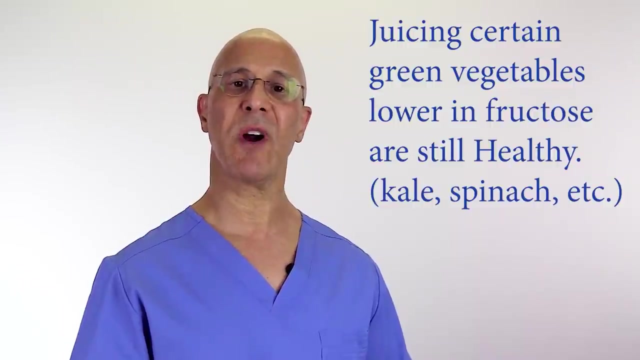 to fall real quick, And this puts a burden on cortisol as well as other hormones within our body. So here's my final answer: I believe that smoothies are healthier from a physiological point of view as compared to juicing, Although juicing will have more concentration. 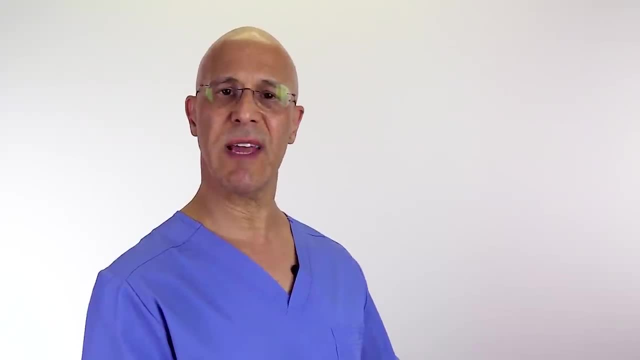 you're going to get a much more concentrated amount of nutrients, But although you still can get plenty of nutrients from the whole state of the fruit or vegetable, my point here is that it's all about the fiber. When you look at heart disease, cardiovascular disease, clogging of the, 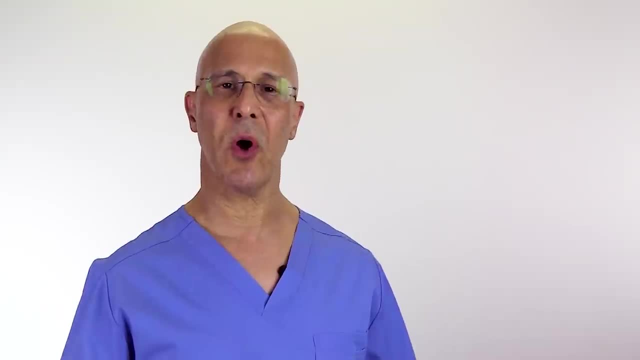 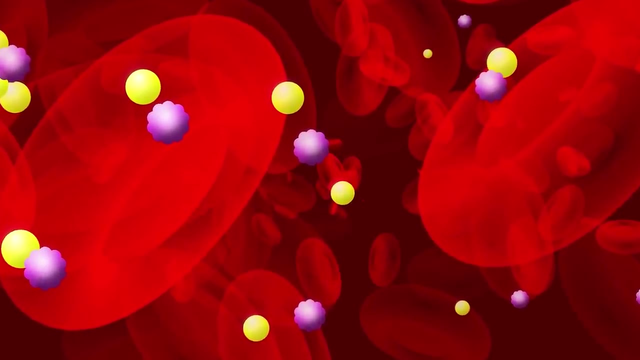 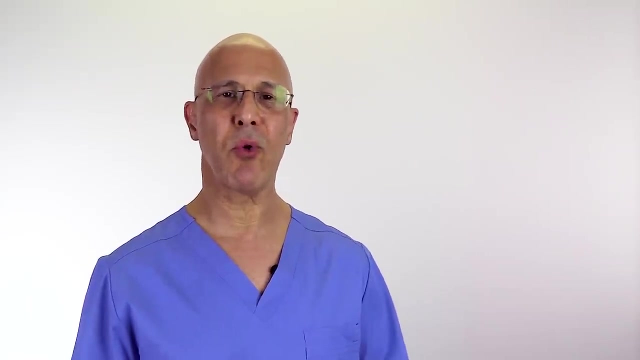 arteries, inflammation, autoimmune problems, diabetes. it's all related to increased spike of those sugars and imbalances of insulin levels. So remember that too much insulin in the body will increase more fat. By all means, fiber is one of the most important things that we can put in.